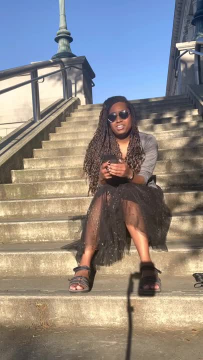 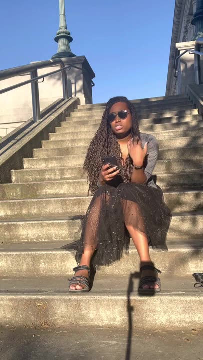 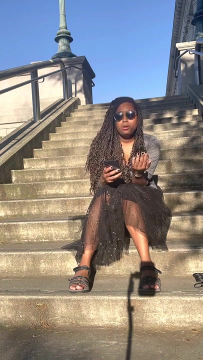 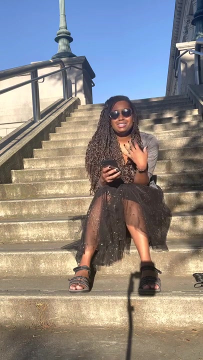 Because, yeah, I guess I want to produce more content that's around the field that I'm actually in, And kind of like walk you guys through my learning process, because I don't just like pop up day one and understand all this stuff about meta learning or AI or ML or engineering. It takes quite some time. The first time I read it it definitely doesn't make any sense. It takes, you know, talking with other people, reading the blog posts, examining the code base, to understand it. 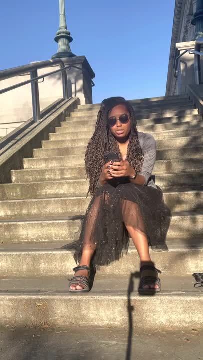 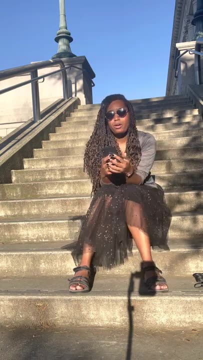 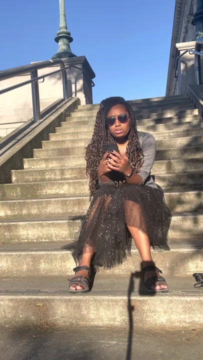 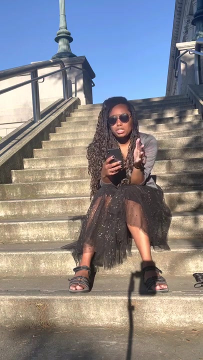 And so we're just going to read this over together. It says it's a 22 minute read. I'm probably going to stop in the middle And dissect some of the stuff, So it might even take a little bit longer, But let's go. So it's called multimodal neurons in artificial neural networks. So we've discovered neurons in CLIP. CLIP is the algorithm that responds to the same concept, whether presented literally, symbolically or conceptually, So that's like different forms of information. That's really interesting. That's new. 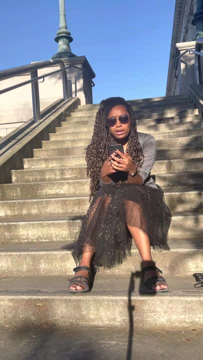 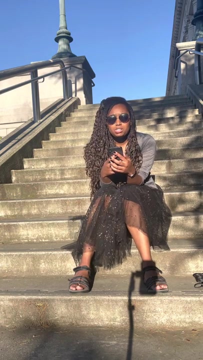 This may explain CLIP's accuracy in classifying surprising visual renditions of concepts and is also an important step toward understanding the associations and biases that CLIP and similar models learn from. So I remember a while ago- well, I actually wasn't that long, It was maybe like six months ago, It might have been longer than that, It might have been a year ago, I can't remember exactly. But Chris Ola started writing about trying to understand like individual neurons in like a deep learning. 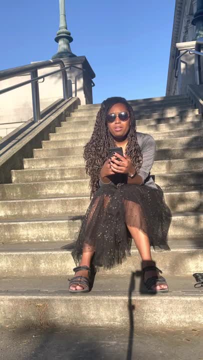 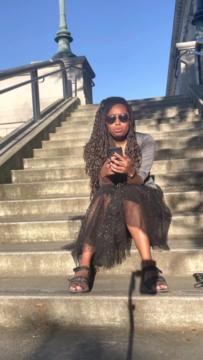 granules, moi, affine, and was writing about that a little bit. I might get those concepts a bit confused, Anyway, so I think this is like buildings directly off of his learning. Okay, so 15 years ago He, Kurosuke et al, discovered that the human brain possesses multimodal neurons. These neurons respond to clusters of abstract concepts centered around a common love. high level theme. 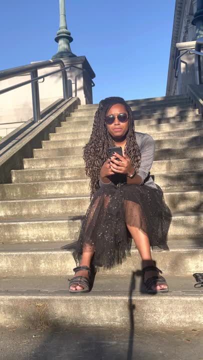 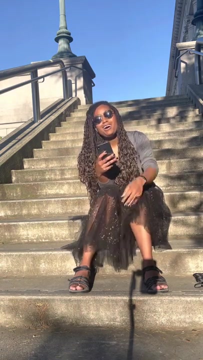 rather than any specific remit than any specific remit, specific visual feature. The most famous of these was the Halle Berry neuron, a neuron featured in both Scientific American and the New York Times. I've never heard of that before. That responds to photographs, sketches and the text Halle Berry, but not other names. 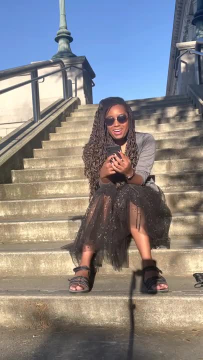 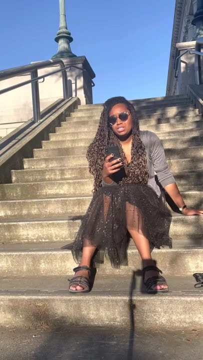 That's funny. Two months ago, OpenAI announced Clip, a general-purpose vision system that matches the performance of a ResNet-50, but outperforms existing vision systems on some of the most challenging data sets. That's kind of cool. ObjectNet ImageNet rendition. 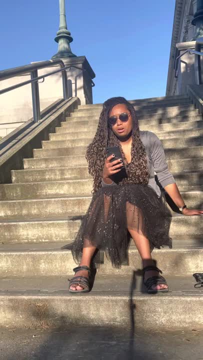 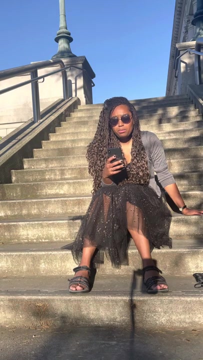 and ImageNet sketch, stress tests and the model's robustness to not recognizing just simple distortions or changes in the lighting or pose, but also to complete abstraction and reconstruction: sketches, cartoons and even statues. Okay, Now we're releasing our discovery of the presence of multimodal neurons in Clip. 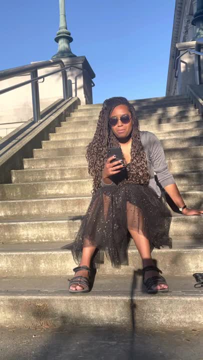 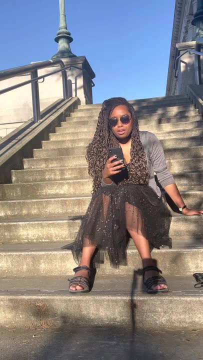 One such neuron, for example, is the Spider-Man neuron, bearing a remarkable resemblance to the Halle Berry neuron. that responds to an image of a spider, an image of the text spider in the comic book Spider-Man, either in costume or illustrated. That's pretty cool. 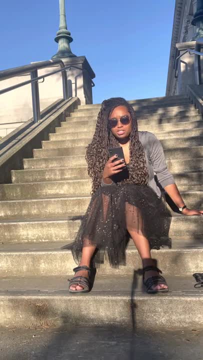 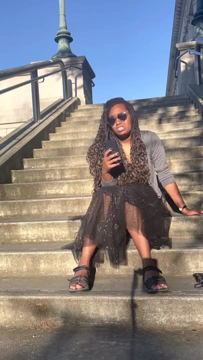 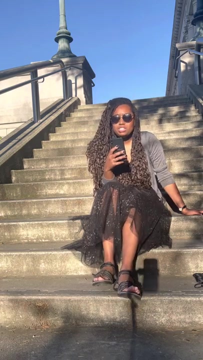 Our discovery of multimodal neurons in Clip gives us a clue as to what may be the most common mechanism of both synthetic and natural vision systems' abstraction. That's interesting. We discover that the highest layers of Clip organize images as a loose semantic collection of ideas, providing a simple explanation for both the model's versatility and the representation's. 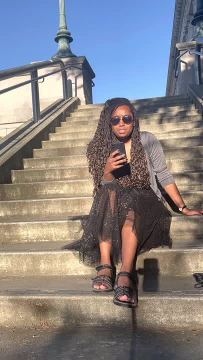 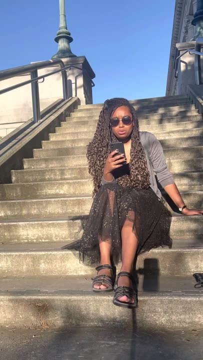 compactness, So it has some images here. Oh, I guess this one is the Halle Berry neuron. It's a biological neuron. The Clip neuron is a biological neuron. The Clip neuron is a biological neuron. The Clip neuron and previous artificial neurons. 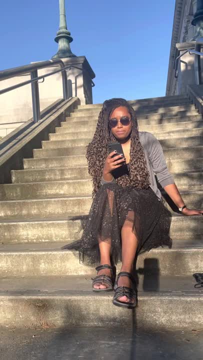 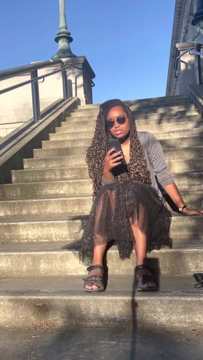 Okay, so it's giving examples of both and what these systems can detect. That's cool. Using the tools of interpretability, we give an unprecedented look into the rich visual concepts that exist within the weights of Clip. Within Clip, we discover how pixels and dua-gase are oriented To help us learn how demographics 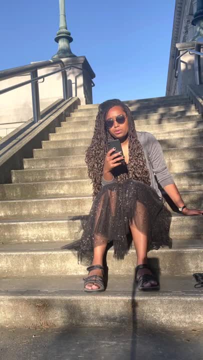 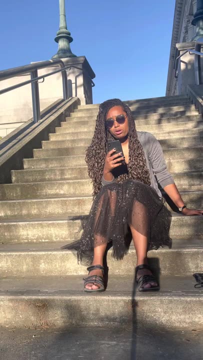 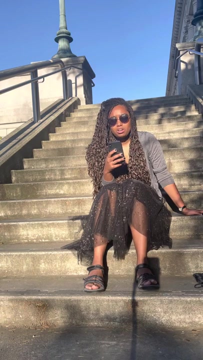 We cover high-level concepts that span a large subset of the human visual lexicon: geographical regions, facial expressions, religious iconography, famous people and more. By probing what each neuron affects downstream, we can get a glimpse into how CLIP performs its classification. 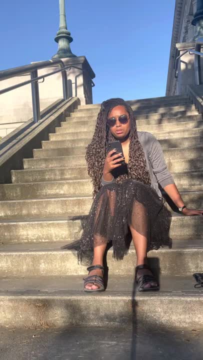 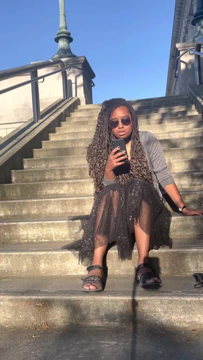 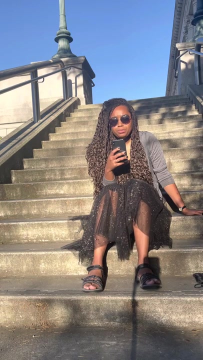 Multimodal Neurons in CLIP. Our paper builds on nearly a decade of research into interpreting convolutional neural networks, beginning with the observation that many of these classical techniques are directly applicable to CLIP. We employ two tools to understand the activations of the model. 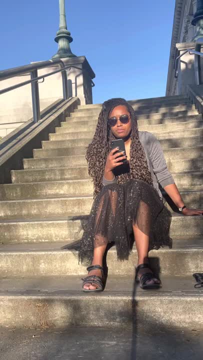 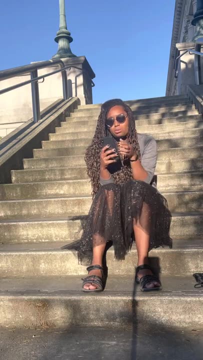 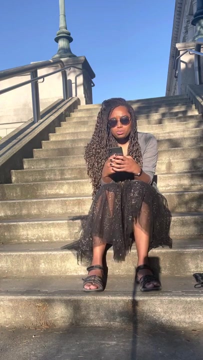 Feature visualization which maximizes the neuron's firing by doing gradient-based optimization on the input and dataset examples, which looks at the distribution of maximal activating images for a neuron from a dataset. Using these simple techniques, we found the most effective way to interpret convolutional neural networks. 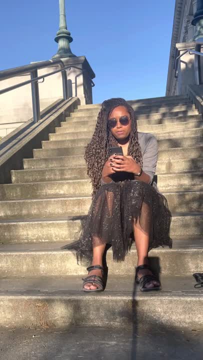 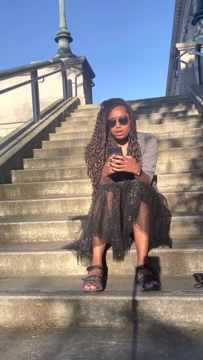 The majority of the neurons in CLIP are in 50 by 4, a resnet 50 scaled up to 4x using the efficient net scaling rule to be readily interpretable. Indeed, these neurons appear to be extreme examples of multifaceted neurons. 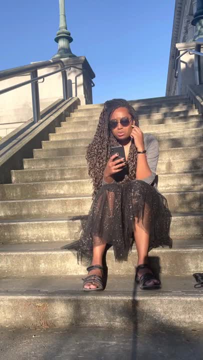 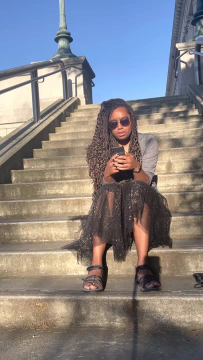 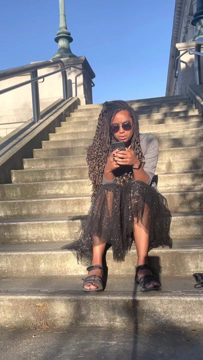 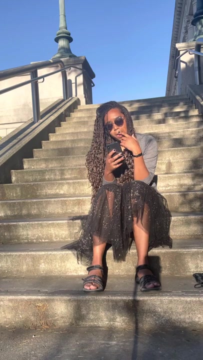 or neurons that respond to multiple distinct cases only at a higher level of abstraction. So they have some categories here. One says summer and I suppose when you query summer, this is what comes up: Summer, winter, shocked mid-1990s, self and relief, Christmas. 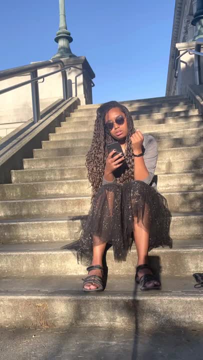 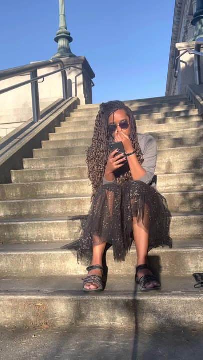 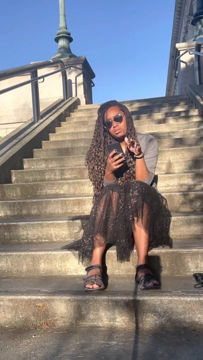 Okay, so for each of these themes they're using the exact same photos, But it's giving Or it's the. The higher level concept is like mid-1990s, but they have. It looks like a different query each time. so, like any text, face logo, architecture, indoor nature, pose. 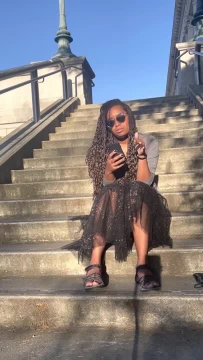 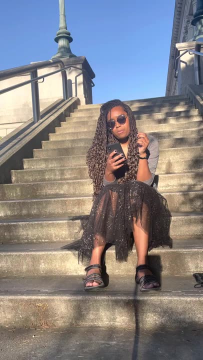 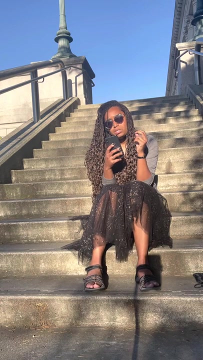 But for whatever the higher level theme is, the pictures change. Roman art, child's drawing, USA, India, heart, West Africa. Selected neurons from the final layer of our CLIP models. Each neuron is represented by. Each neuron is represented by a feature visualization with a human-chosen concept, labels to help quickly provide a sense of each neuron. 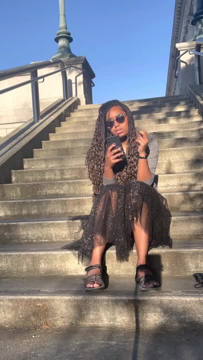 Okay labels were picked after looking at hundreds of stimuli that activate the neuron. in addition to feature visualizations, We chose to include some of the examples here to demonstrate the model's proclivity towards stereotypical depictions of regions, emotions and other concepts. 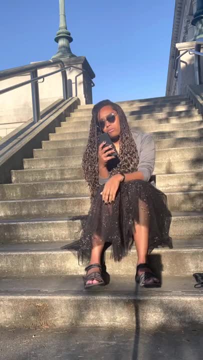 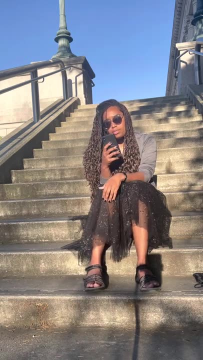 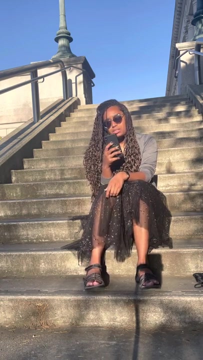 We also see discrepancies in the level of neuronal resolution. while certain countries like the US and India were associated with well-defined neurons, The same was not true of countries in Africa, where neurons tended to fire for entire regions. We discussed some of these biases and their implications in later sections. 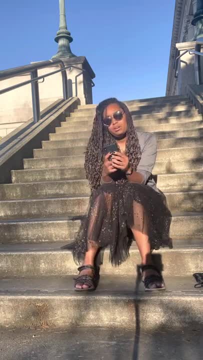 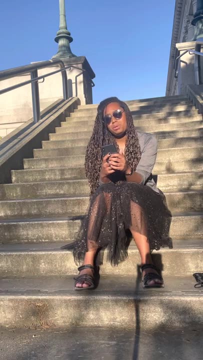 Oh, that's interesting. Well, I guess, when you think about it, whatever's like widely tagged on the internet is probably American, And People do talk about Africa as like an entire continent when there are so many countries in Africa. so I guess that makes sense. 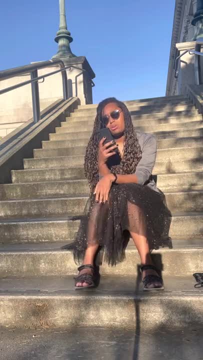 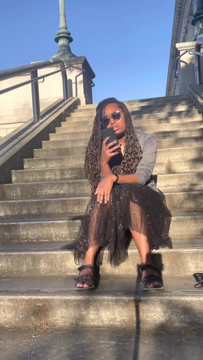 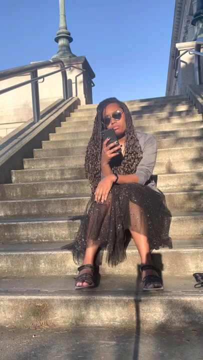 Indeed, we were surprised to find many of these categories appear to mirror neurons in the medial temporal lobe documented in epilepsy patients with intracranial depth electrodes. These include neurons that respond to emotions, animals and famous people, But our investigation into CLIP reveals many more such strange and wonderful abstractions. 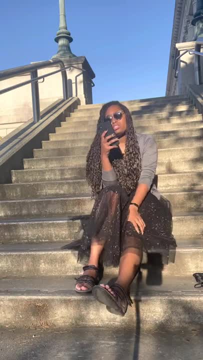 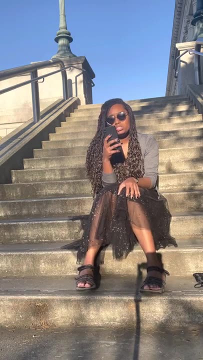 including neurons that appear to count, neurons responding to art styles, even images with evidence of digital alteration. Absent Concepts. While this analysis shows a great breadth of concepts, we note that a simple analysis on a neuron level cannot represent a complete documentation of the model's behavior. 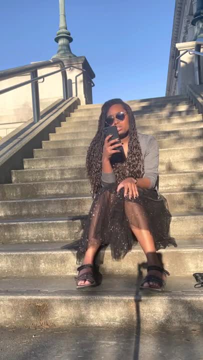 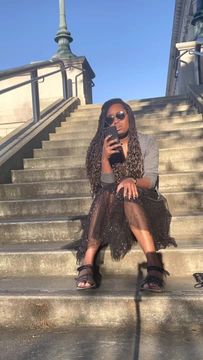 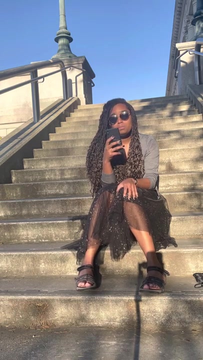 The authors of CLIP have demonstrated, for example, that the model is capable of very precise geolocation, With a granularity that extends down to the level of a city and even a neighborhood. In fact, we offer an anecdote: We've noticed, by running our own personal photos through CLIP, that CLIP can often recognize if a photo was taken in San Francisco, and sometimes even the neighborhood, like Twin Peaks. 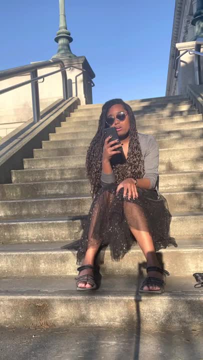 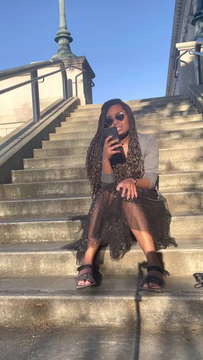 Despite our best efforts, however, we have not found a San Francisco neuron. nor did it seem from attribution that San Francisco decomposes knives and knives. It decomposes nicely into meaningful unit concepts like California and a city. That's interesting. We believe this information to be encoded within the activations of the model somewhere, but in a more exotic way, either as a direction or some other more complex manifold. 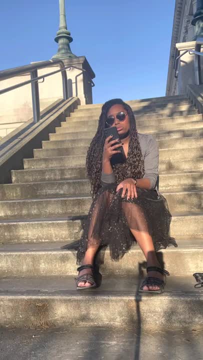 We believe this to be a fruitful direction for further research How Multimodal Neurons Compose. These multimodal neurons can give us insight into understanding how CLIP performs classification. With a sparse linear probe we can easily inspect CLIP's weights to see which concepts combine to achieve a final classification for ImageNet classification. 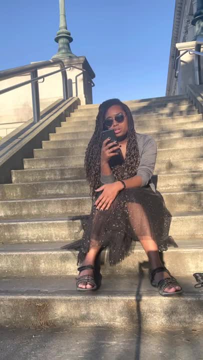 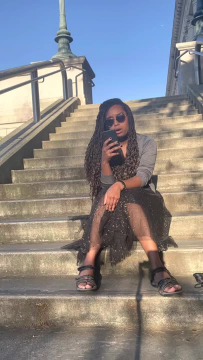 Hmm, So there's an image labeled piggy bank, an image labeled finance. we've got dolls and toys, barn spider, Oh okay. so we've got like piggy bank equals finance, which has a weight of 2.5, and then dolls and toys, which has a weight of 1.1.. 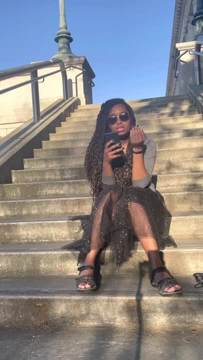 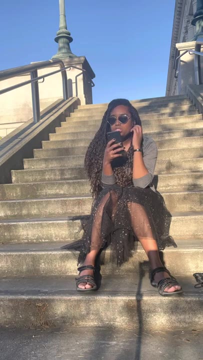 And they're saying you combine those to get like the piggy bank image. That makes sense. So then you have like a weight of 2.9 given to an image- spider-man- 1.5 given to animal. 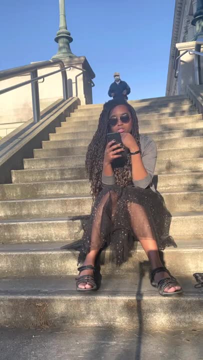 You add those and you get like barn spider. So the piggy bank class appears to be a composition of the final classification. So the piggy bank class appears to be a composition of the final classification. So the piggy bank class appears to be a composition of the final classification. 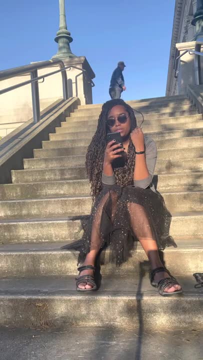 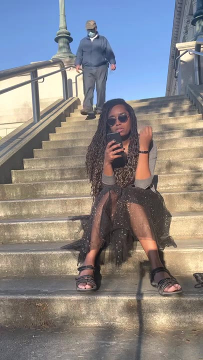 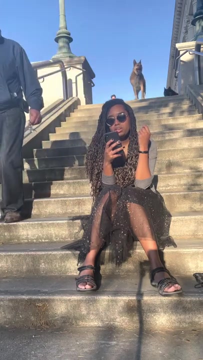 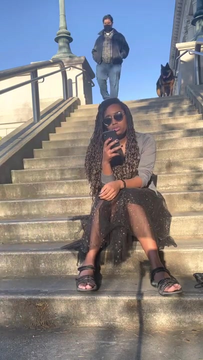 Similar to the finance neuron. along with the porcelain neuron, the spiderman neuron referenced in the first section of the paper is also a spider detector and plays an important role in the classification of the class barn spider. For a text classification, a key observation is that these concepts are contained within neurons in a way similar to the word-to-vect objective is almost linear. 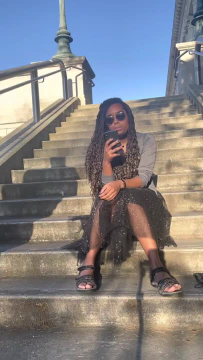 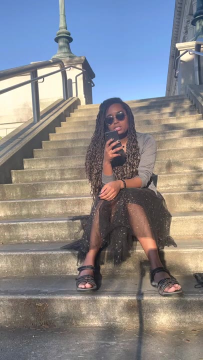 The concepts therefore form a simple algebra that behaves similarly to a linear probe. By linearizing the attention, we too can inspect any sentence, such as a linear probe, as shown below, So probing how Clip understands words. it appears to the model that the word 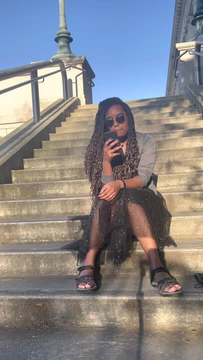 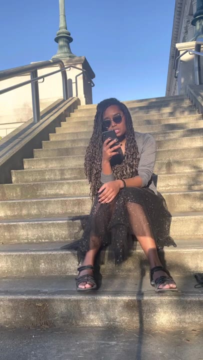 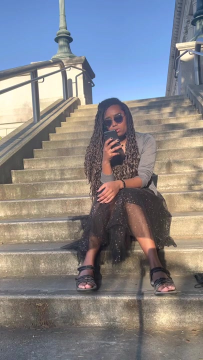 surprise implies some kind of measure of shock, but a shock of a very specific kind, one combined perhaps with delight or wonder. Intimate consists of a soft smile and hearts, but not sickness. We note that this reveals a reductive understanding of the full human experience of intimacy. 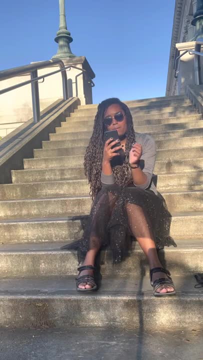 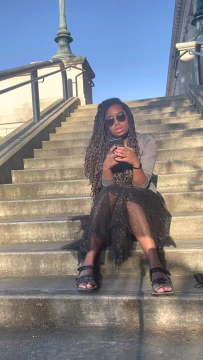 The subtraction of illness precludes, for example, intimate moments with loved ones who are sick. We find many such omissions when probing Clip's understanding of language, Fallacies of Abstraction, The degree of abstraction in Clip surfaces a new vector of attack that we believe is not manifested in previous systems. 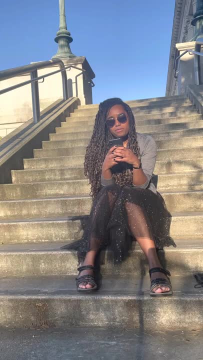 Like many deep networks, the representations of the highest level of the model are completely dominated by such high-level abstractions. What distinguishes CLIP, however, is a matter of degree. CLIP's multimodal neurons generalize across the literal and iconic, which may be a double-edged sword. 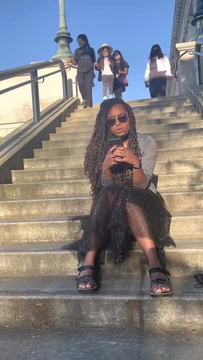 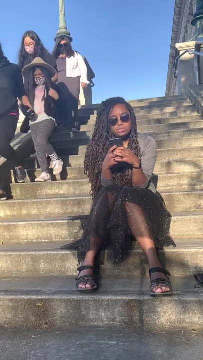 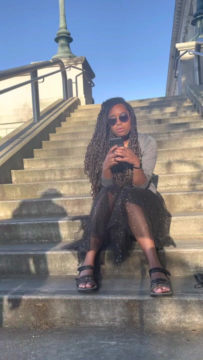 Through a series of carefully-constructed experiments, we demonstrate that we can exploit this reductive behavior to fool the model into making absurd classifications. We've observed that the excitations of the neuron in CLIP are often controllable by its response to images of text, providing the simple vector of attacking the model. 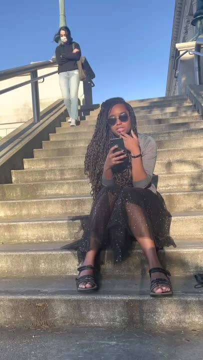 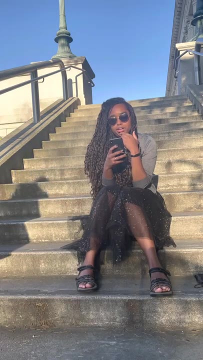 The finance neuron, for example, responds to images of piggy banks, but also responds to the string. It's like these dollar signs. By forcing, let's say, a vector of attack, we can exploit this reductive behavior. By forcing the finance neuron to fire, we can fool our model into classifying a dog as a piggy bank. 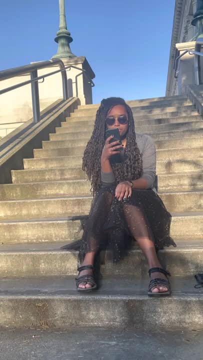 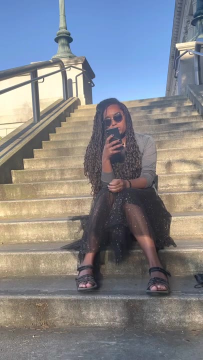 Oh, that's interesting, Huh Huh. so the standard poodle had a classification rate of like 39.3%, and then it looks like in the—wait. let's just read the caption. So by rendering text on an image, we artificially stimulate neuron—. 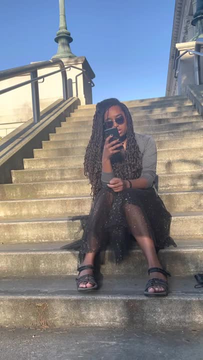 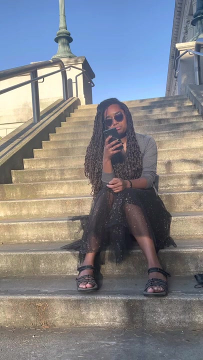 1330, which has a high weight into the class piggy bank, in a linear probe. Oh, so they put all of these like image markers, those text markers on the poodle, and so that's—because those text markers had like, um, almost like a direct correlation to that piggy bank label, that piggy bank classifier. 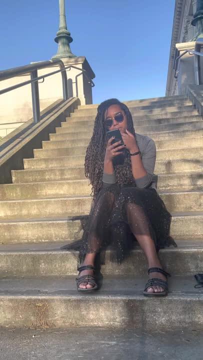 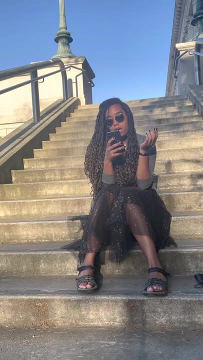 And once that like text was added to the image- uh, the classification— the classification went from standard poodle at 39.3% to piggy bank at 52.5%, and the second highest classification was a standard poodle. 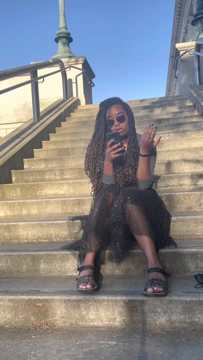 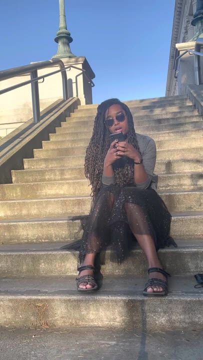 So that's—I mean, that's kind of interesting. I didn't think of that. That's—that's actually really cool. Uh, so attacks in the wild. We refer to these attacks as typographic attacks. We believe that such attacks, such as those described um above, are far from simply an academic concern. 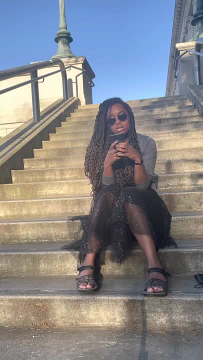 By exploiting the model's ability to read text robustly. we find that even photographs of handwritten text can often fool the model. Like the adversarial patch, this attack works in the wild, but, unlike such attacks, it requires no more technology than pen and paper. 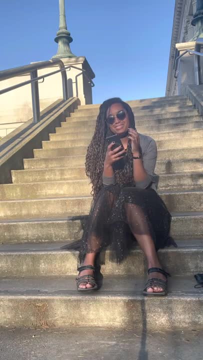 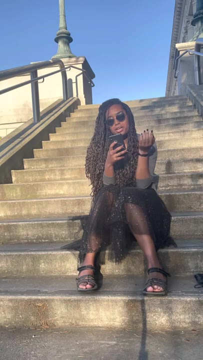 Oh, this is funny. So they have an apple on the table and, uh, the regular classifier is like it's 80—85.6% positive, it's a Granny Smith apple. but then they put a label that just says: like iPod. 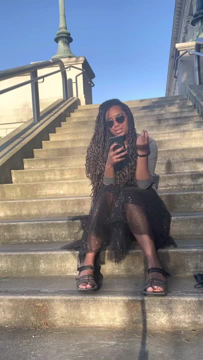 And then it's like 1%- sure it's a Granny Smith apple and 99.7% sure it's an iPod. That's funny: When we put the label saying iPod on this Granny Smith apple, the model erroneously classifies it as an iPod on the zero-shot setting. 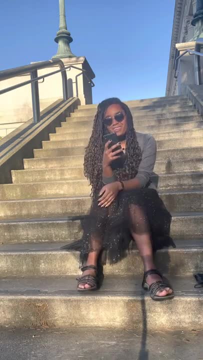 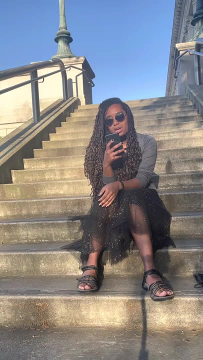 That's cool. Oh, We also believe that these attacks may also take a more subtle, less-conspicuous form. An image given to CLIP is abstracted in many subtle and sophisticated ways, and these extractions may over-extract common patterns, over-simplifying and, by virtue of that, over-generalizing. 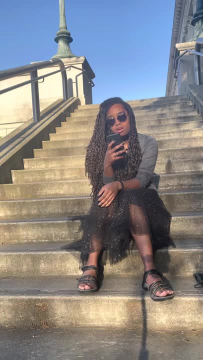 Okay, so now we're at bias and over-generalization. Our model, despite being trained on a curated subset of the Internet, still inherits its many unchecked biases and associations. Many associations we have discovered appear to be benign, but yet we have discovered several cases where CLIP holds associ—.